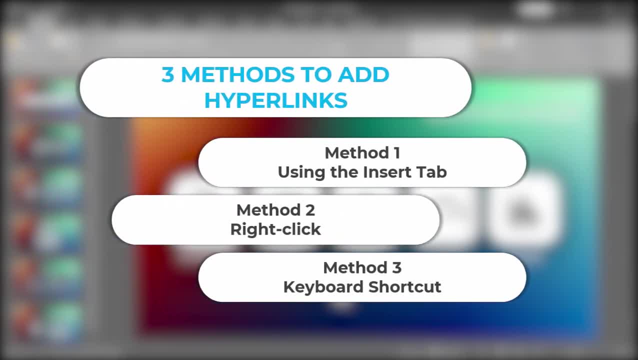 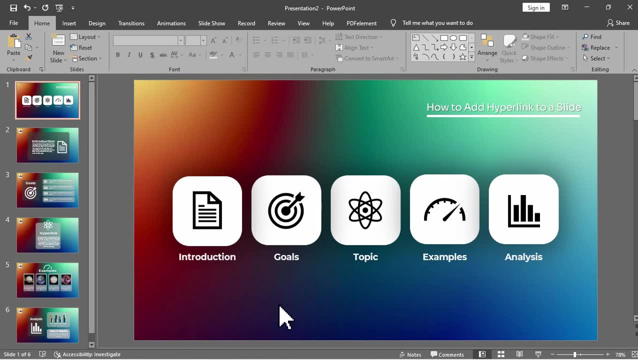 to slide. In this video I will show you the three methods on how you can add hyperlinks between slides from the same file in Microsoft PowerPoint. The first method is by selecting the element to which you want to add a hyperlink. Let's try this: introduction icon first, then under the insert: 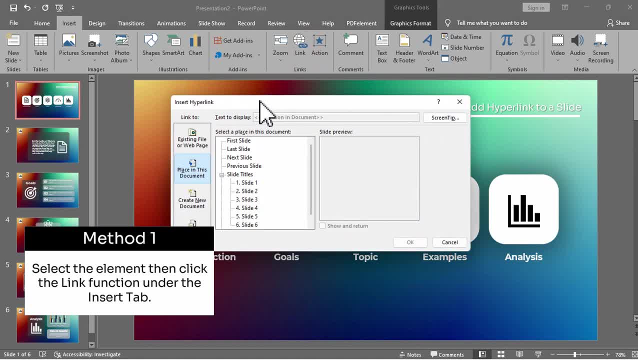 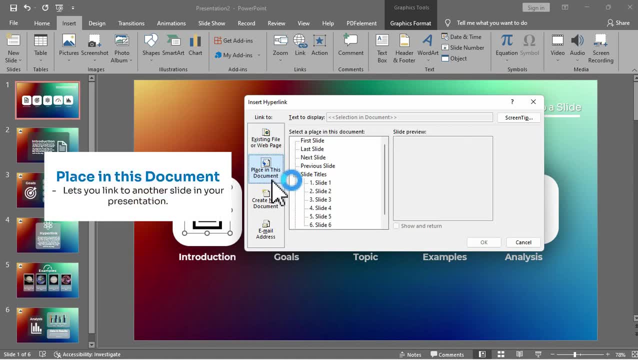 tab. we will click the link function. You will see that the link function is added And you will. You will see four tops in the dialog box that appears: the existing file or web page option, the place in this document option and these two options below. 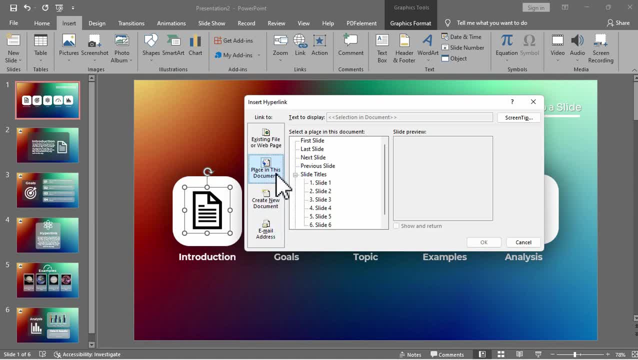 In this tutorial we will just use the second option or the place in this document option. Then you will be given a choice on which slide you want to land or direct us. whenever you click that icon, You can choose the first, last and next, or select a particular slide from the presentation. 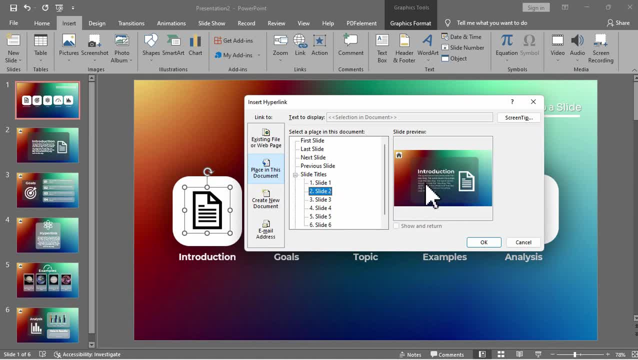 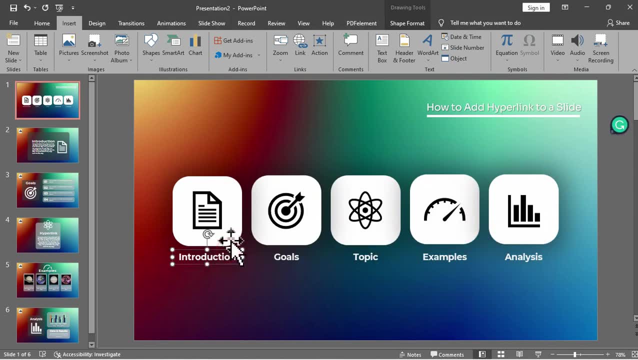 Since this icon represents the introduction part, I will select the slide corresponding to the introduction slide, which is the slide 2.. We can also add a hyperlink function to text using the same method. Let us see the preview so far. So whenever we click this icon and text, it will automatically go to the slide 2 or the 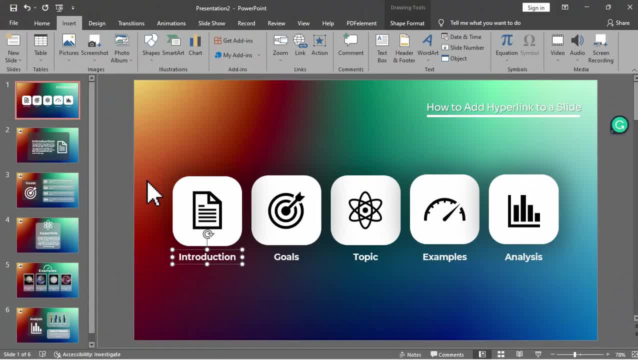 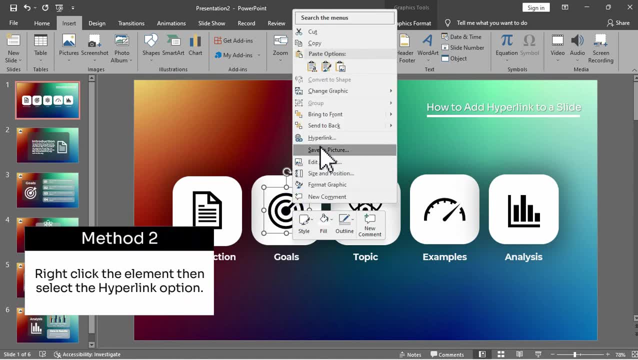 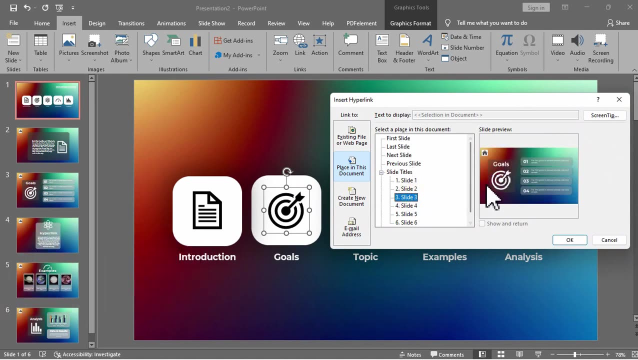 introduction slide. Now for the second icon and text. We will use the slide 2.. We will use the second method by right-clicking the element we want to hyperlink and then click the hyperlink function. Same as we did earlier. we will select our desired slide, which in this case will be the. 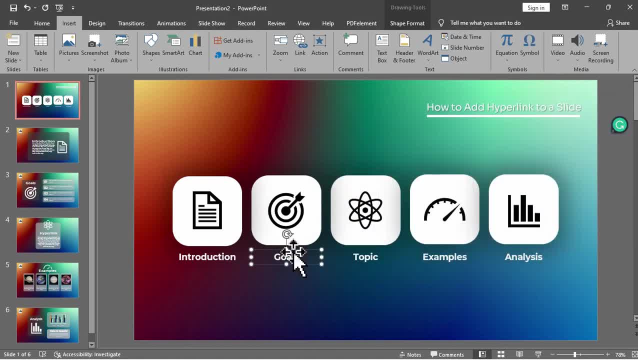 third slide, or the gold slide, We will also add a hyperlink to the text title under this icon. If ever you want to change the hyperlink settings, just right-click the element again and select the edit link option. Now for our third icon. We will use the third method by using a keyboard shortcut: Ctrl plus K. 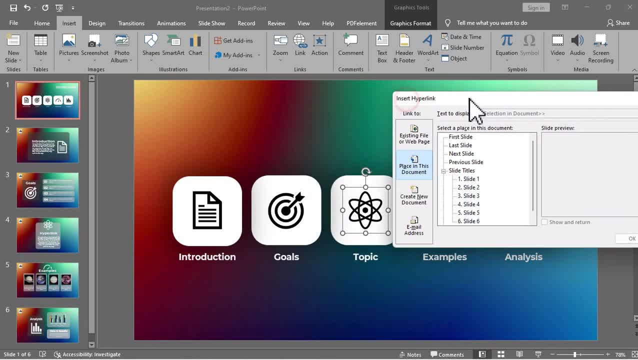 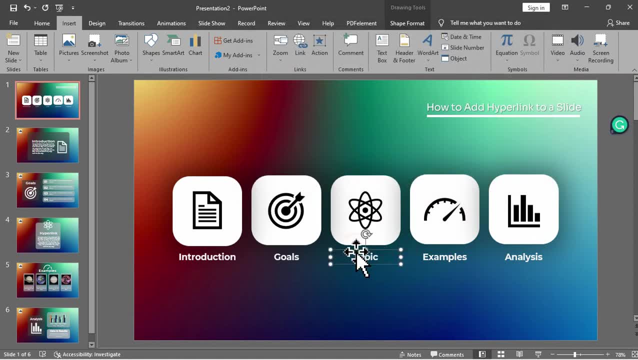 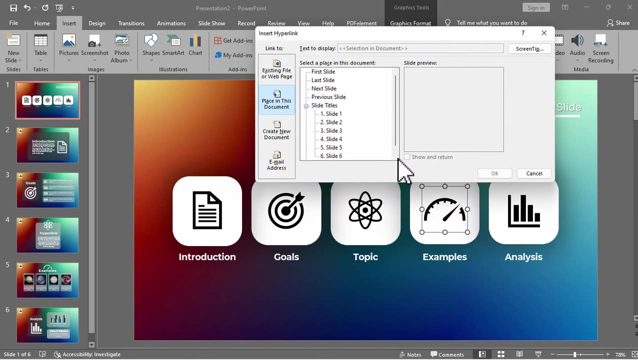 Just select the element and hit Ctrl plus K from your keyboard. Then you can customize your hyperlink in the dialog box. The same thing for the text. we will use the keyboard shortcut function. For the remaining icons, you can decide which method you will use in customizing your hyperlinks.